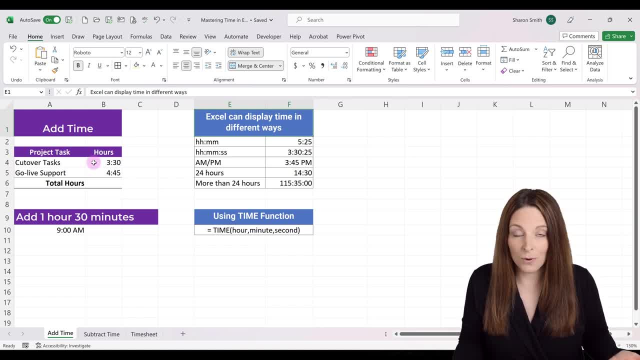 time into Excel. it recognizes it as time, it'll format it a certain way and then we can actually just add it like we normally would to other values in Excel. So if we come over here and we want to sum these two values for our project tasks to figure out, 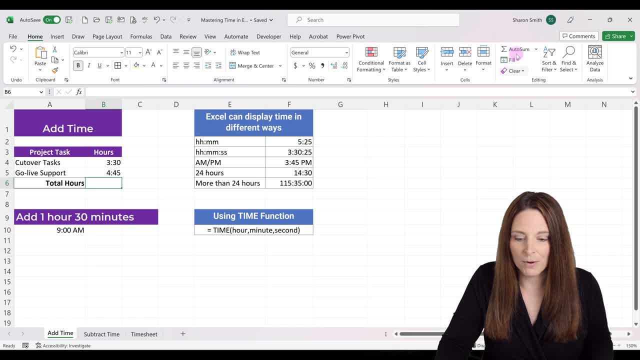 how much time we've spent doing that. all we have to do is come over here on the home tab and click on auto sum and then hit enter, And that's going to give us 8 hours and 15 minutes. Now let's say that we are going to enter time that would exceed 24 hours, So let's just put 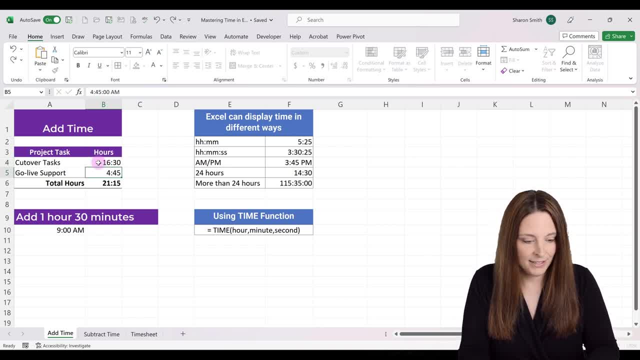 16, 30 and 18, 25.. Now we know that that's more than 10 hours and 55 minutes. so it's how Excel is recognizing the formatting of this cell, So we need to update that. So right click on the cell. 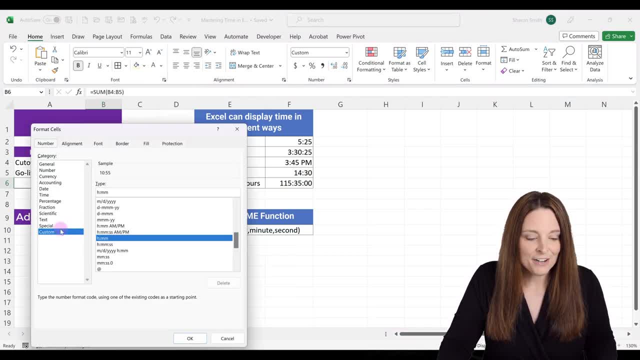 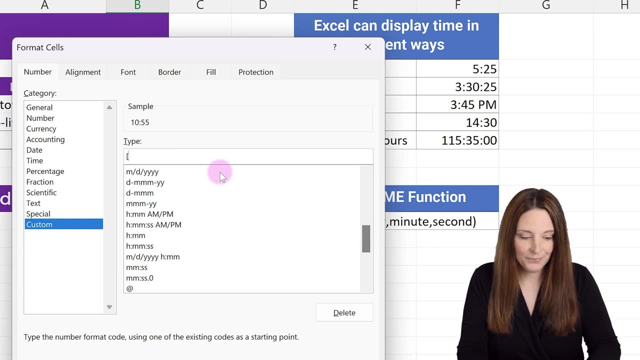 and select on format cells And down here under custom, come over here to type: We're going to select that and we're going to type an open bracket, H, close bracket, colon, mm. And those brackets are telling Excel to allow more than 24 hours in the calculation. 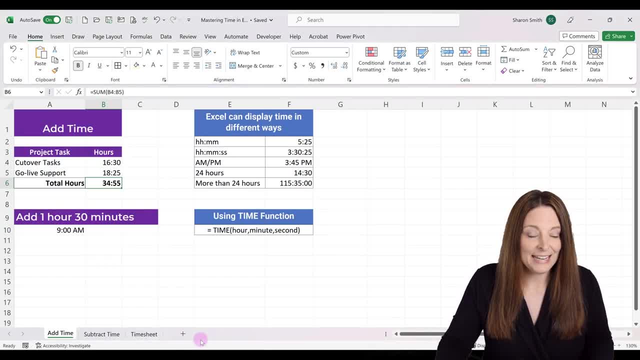 And then we're going to click ok, And now it correctly displays as 34 hours and 55 minutes. So now let's go down here and see how we can use the time function to actually add an amount of time to a certain time. 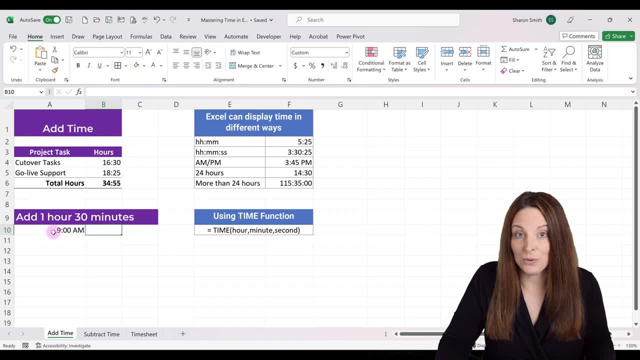 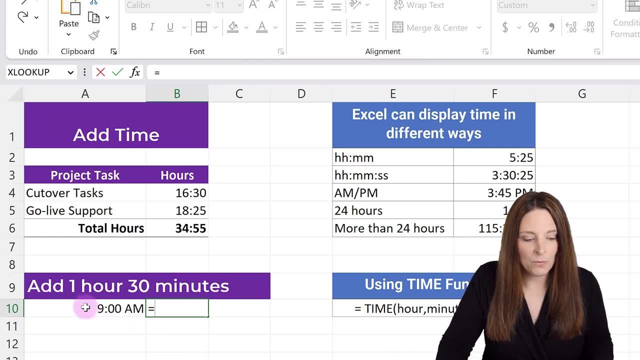 So we want to add an hour and 30 minutes to 9 am. So all we have to do is select our cell hit equals, and then we're going to select the cell that we want to add, And then we're going to say plus and then we're going to insert the time function. 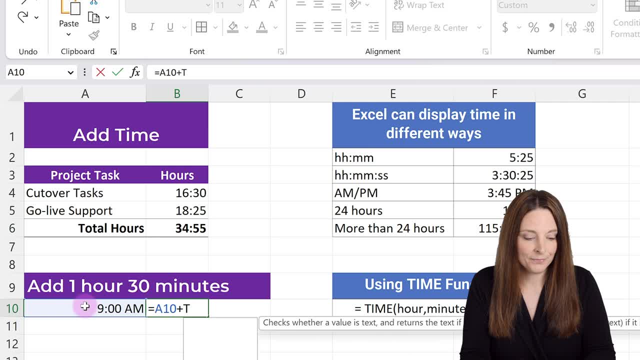 So all we have to do is start typing time And then we open a parenthesis and then the syntax for the time function is hour comma, minute comma, seconds. So we're going to add one hour comma and then 30 for our minutes, comma zero for seconds, and close our parenthesis and hit enter. 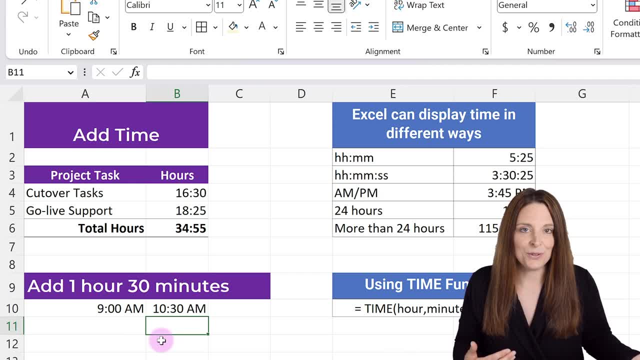 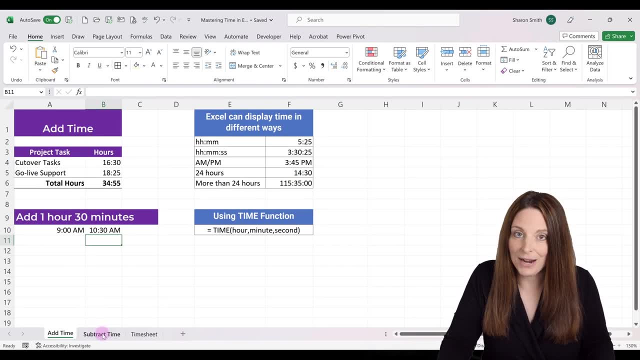 And that gives us 10- 30 am and allows us to use this as a calculator to add time to a specific time that we want to look at Now. let's take a look at how we would subtract time in Excel. Now, when we subtract time in Excel, there's a few things we want to keep in mind. 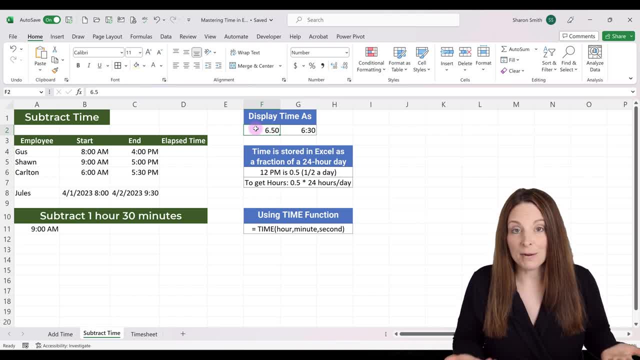 We can display elapsed time as either a number, So this would be displayed as six and a half hours, or as six hours 30 minutes, And we want to display this as a number. So we're going to reformat that after we do our calculation. So let's calculate how much time has elapsed. 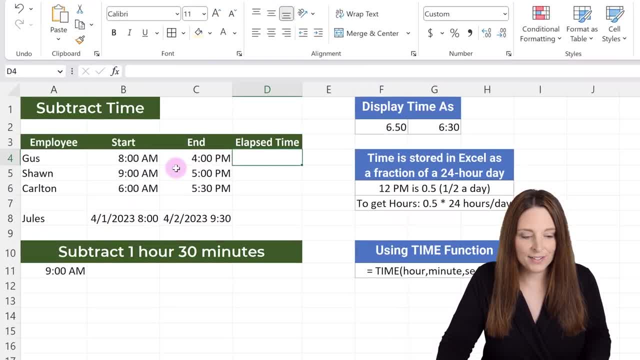 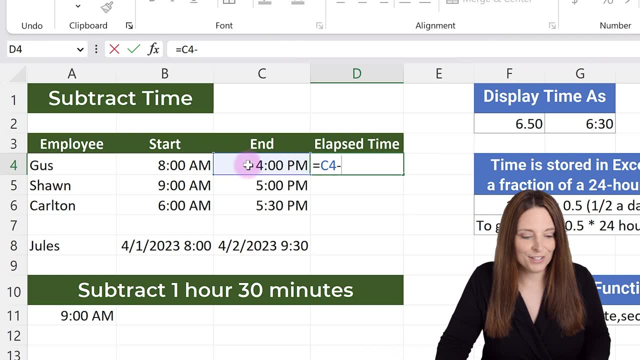 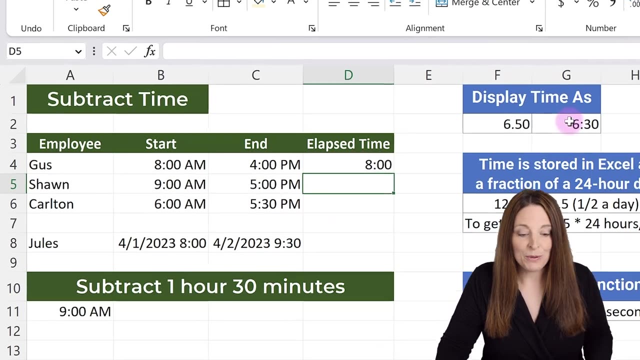 between the ending and starting times over here. So we're going to just select our cell, hit equals, and then we're going to select our end time minus our start time and then hit enter. Now that gives of time, but we want to display this as a number, as a decimal to two spaces. So what we want to 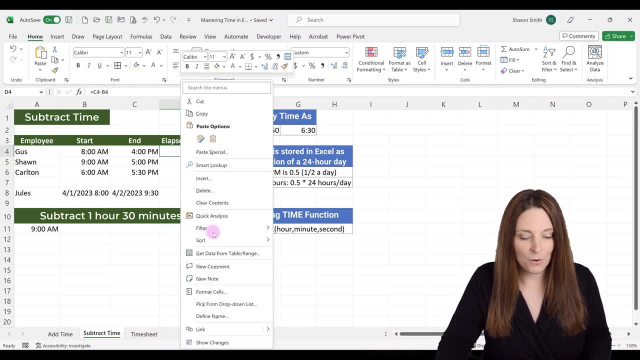 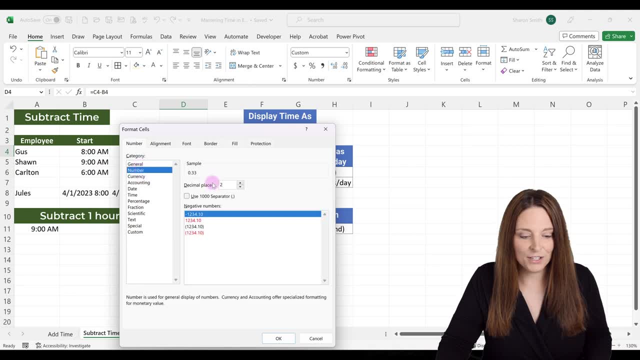 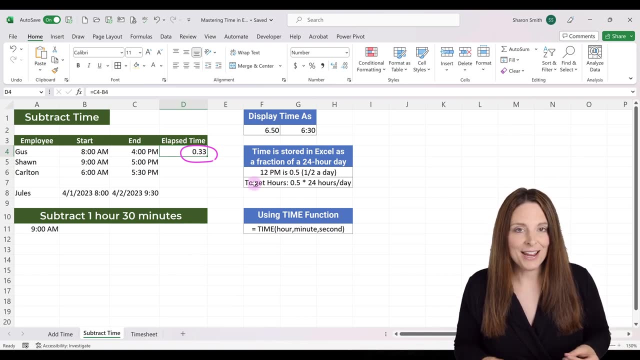 do is select the cell right click, click on format cells and instead of custom, we're going to come up here to number and we have that to two decimals and we're going to click ok. Now notice, that gives us a fraction of time and the reason it's being stored as 0.33 is that Excel is storing this as: 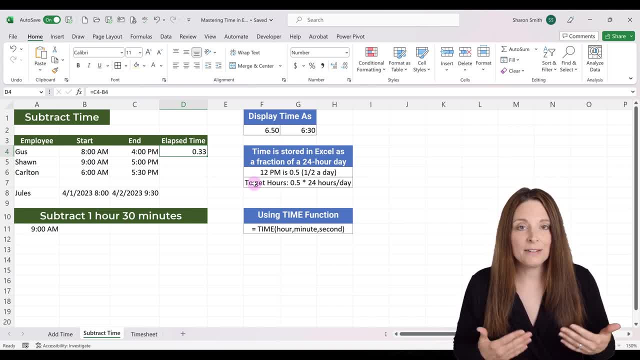 a fraction of a 24 hour day. So to get the correct eight hours of time, we're going to need to multiply this by 24.. So all we have to do is select our cell and we're going to come up into our formula bar. 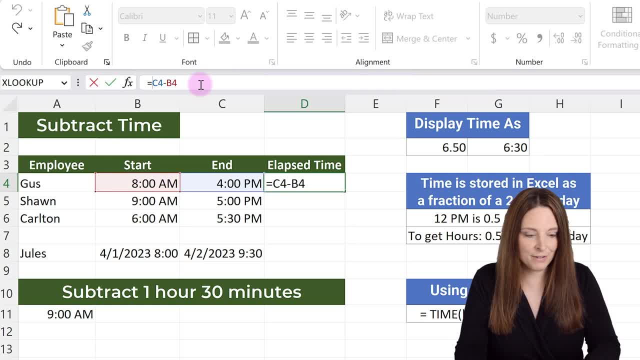 and put parentheses around our formula up here. So the total amount of time that elapsed, we want to multiply that by 24.. So we're going to say asterisk 24 and hit enter and that's going to give us 8.0, the eight hours of time. So we're going to go back to our formula bar and we're going to 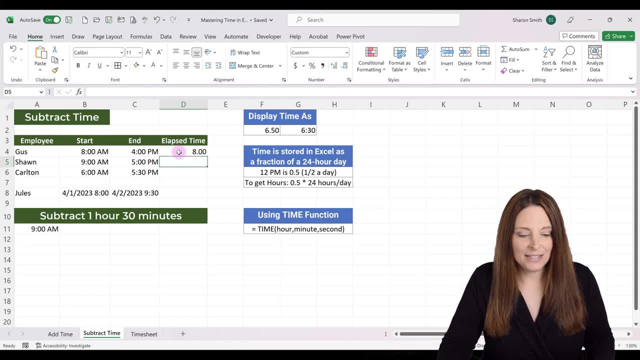 select the cell that we want to display Now. then all we have to do is copy that formula down and it will retain all of the formatting and it will display: even over 24 hours will display correctly as 25.5 hours Now, just like we did when we added time using the time function. we can also subtract. 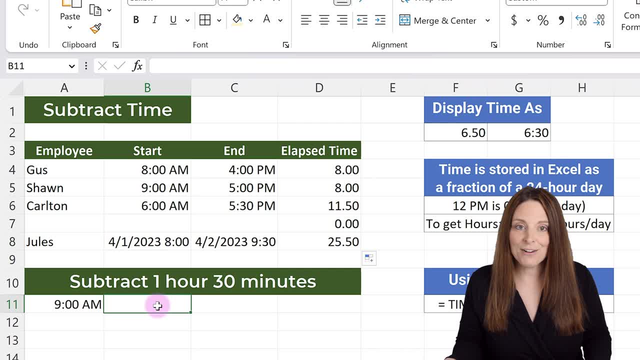 time using the time function. So if we want to subtract an hour and a half from a time, all we have to do is hit equals, select the cell with the time minus, and then we're going to have a time function and then we put the time function. So start typing time. open parentheses: 1,30,0. 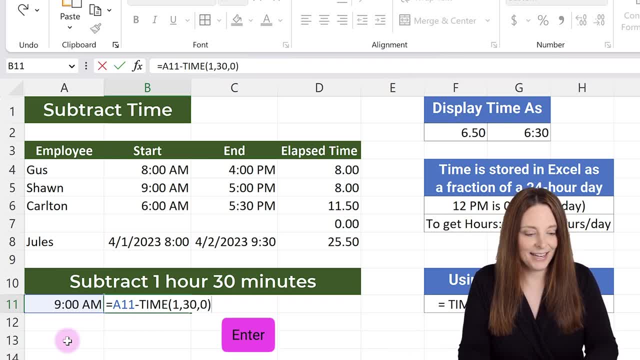 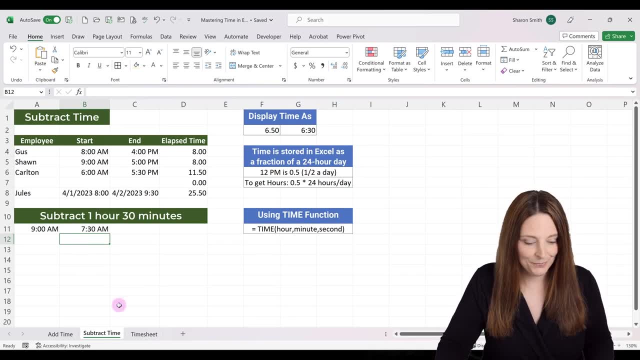 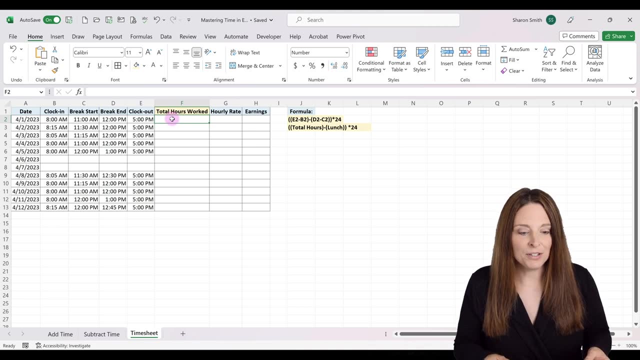 for seconds and close the parentheses and hit enter, And that gives us our calculated time of 7.30.. Now let's move on to our timesheet example. Okay, so here I want to calculate total hours worked as a number, so that I can multiply that by someone's hourly rate and figure out their. 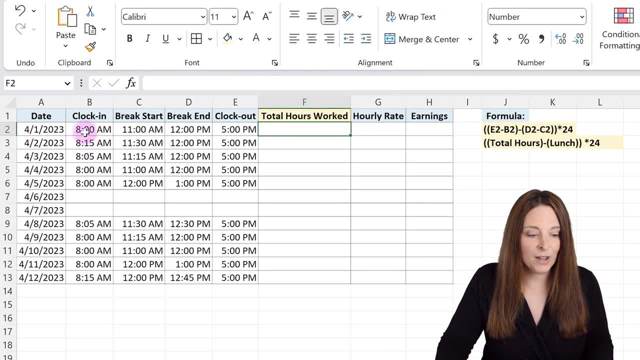 earnings. And so I have here an example of when people clocked in, when they clocked out for the day and then when they took their lunch break. So a clock in and out for their lunch break. So what we want to do, 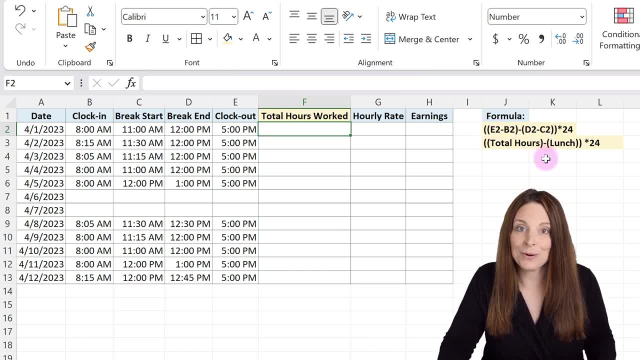 here. I've got the formula over here that explains what we're going to do. But we're basically going to come over, we're going to say equals and then we're going to open up a parentheses and we're going to say the clock out time minus the clock in time. 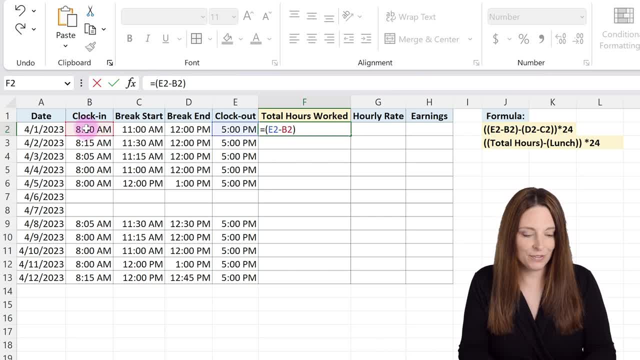 Let me find my clock out and close parentheses. that gives us the total hours worked for the day, But we want to subtract the amount of time that someone was on their lunch break. So we're going to say minus parentheses and then their break end time, minus the break start time and. 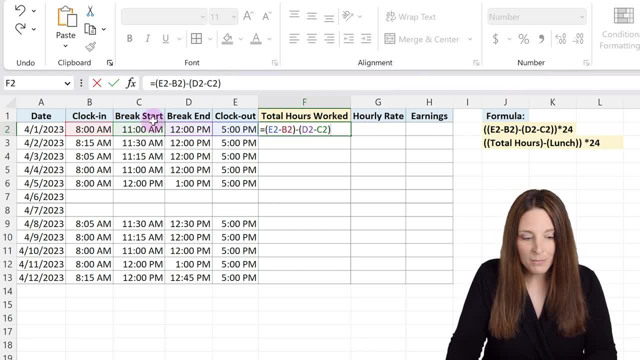 then close those parentheses. Now we want to put parentheses around that entire timeframe there, so we're going to open and close the parentheses at the beginning and end of those two period. Alright, so we now got our total hours and we're going to put parentheses at a moment apart until the�. 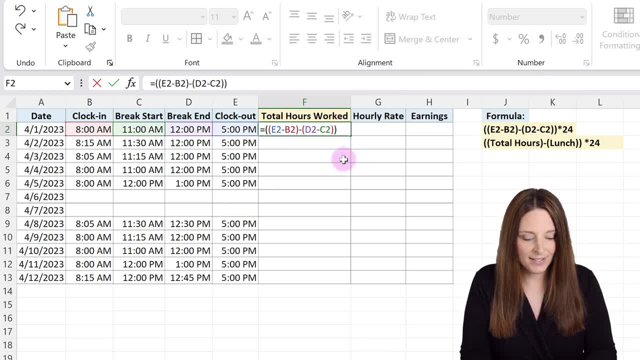 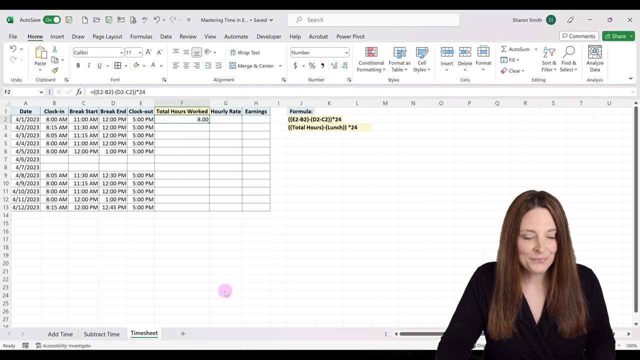 all wonderful hours come by formulas and then we're going to say times 24 and hit enter and that's going to give us our total hours worked and we can always right-click select format cells and make sure that that is formatted as the number that we want. and 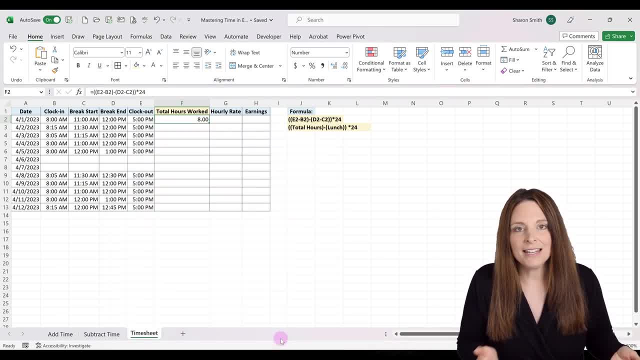 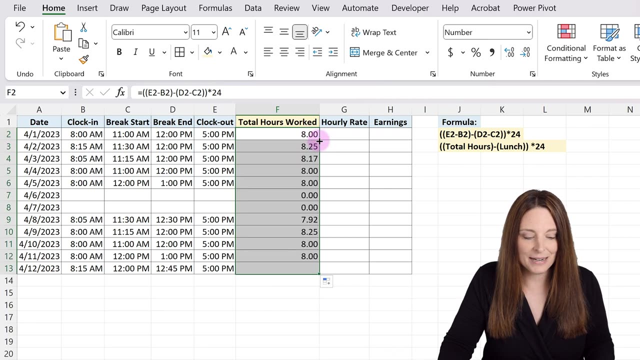 click OK. now if we had left this calculated as as time, as an hour of time, then we may not be able to multiply that successfully to get their earnings. so that's why we want this to be represented as a number, and then all we have to do is copy that all the way down by double clicking, and then we can.